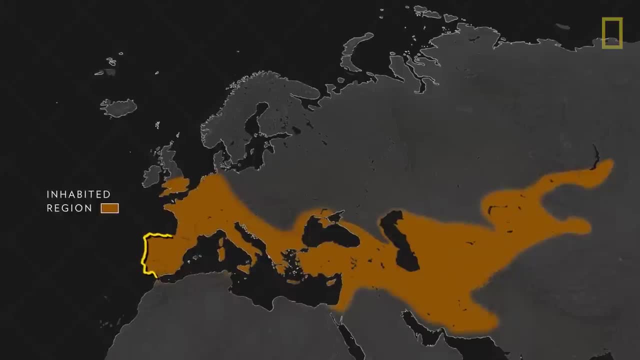 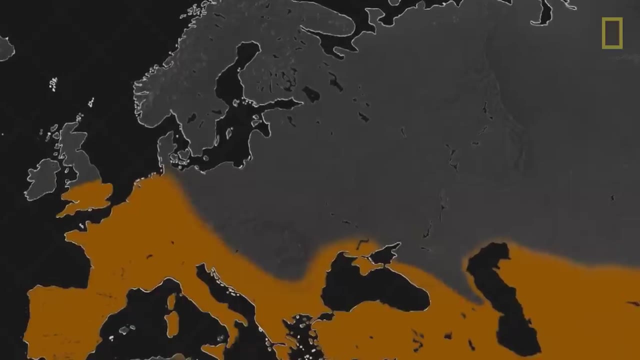 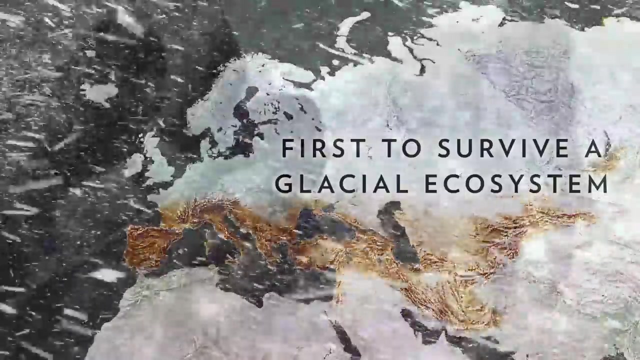 and inhabited an area that stretched as far west as Europe's Atlantic coast and as far east as Central Asia. Their habitat reached northward to modern-day Belgium, making them the first humans to survive a cold glacial ecosystem. The north's cold environment may have influenced Neanderthals' physique. 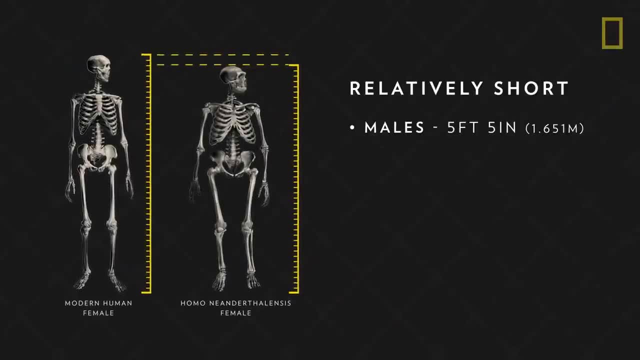 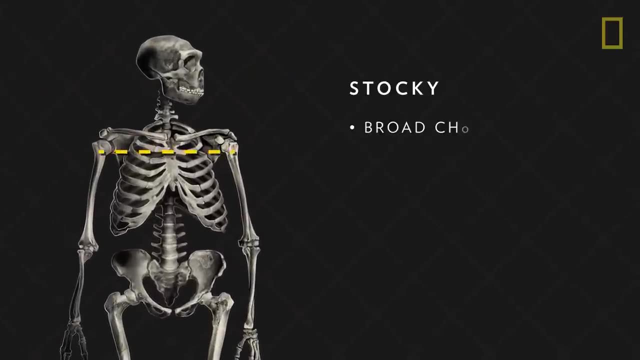 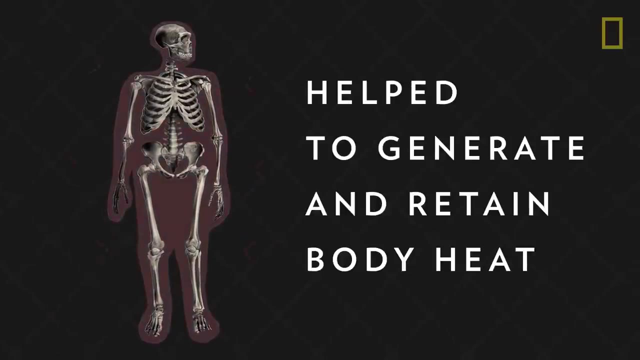 Their bodies were relatively short, with males averaging 5 feet 5 inches and females 5 feet 1 inch tall, And they were stocky, with broad chests, bulky torsos and muscular limbs. These adaptations helped Neanderthals generate and retain body heat. 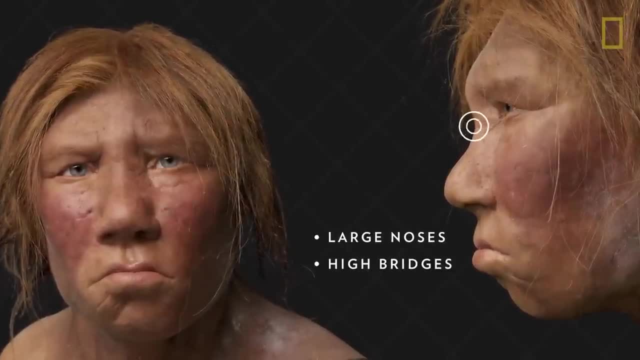 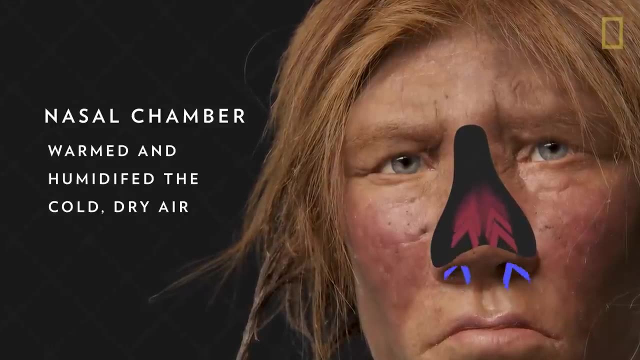 Also, their noses were large and had relatively high bridges. This created a nasal chamber that warmed and humidified the cold, dry air they'd breathe in northern regions. Apart from adaptations that helped Neanderthals survive a harsh, wintry habitat, 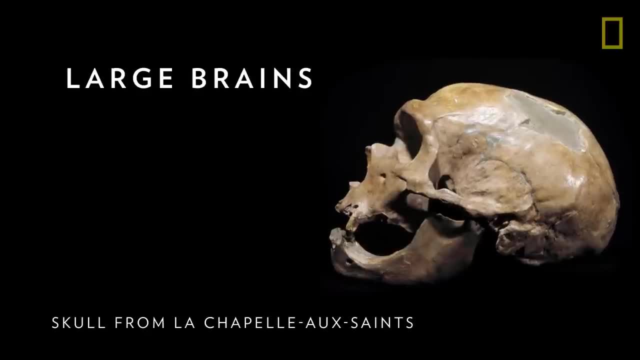 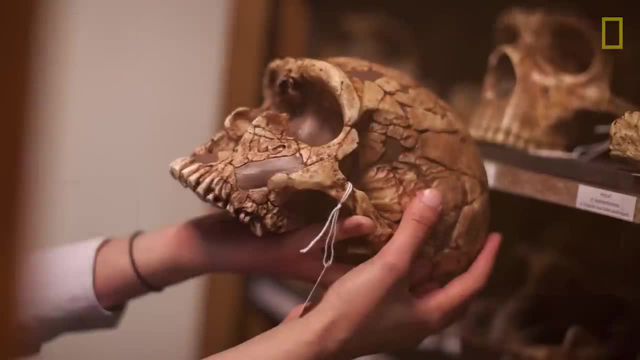 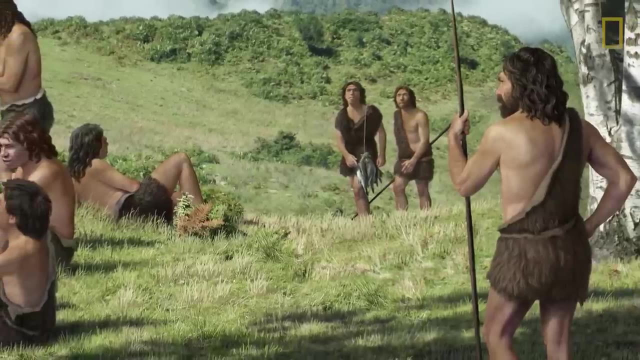 the species also developed a natural habitat and large brains. They were similar in size to modern humans' brains and were often larger. An increase in brain size may have played a significant role in another type of adaptation: Culture. Culture is indicative of an intelligent species. 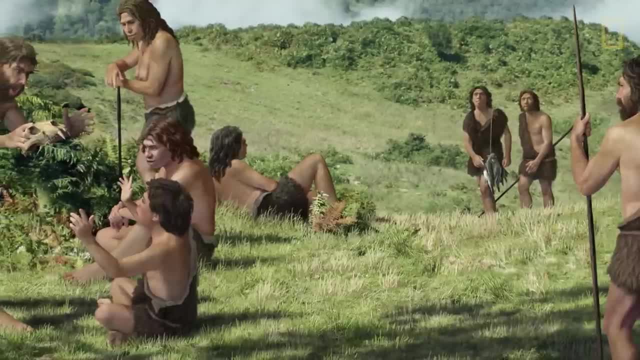 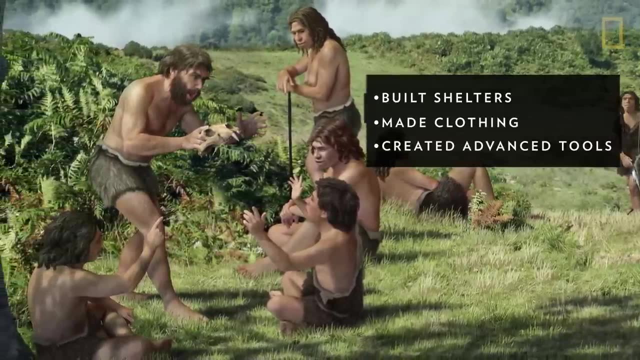 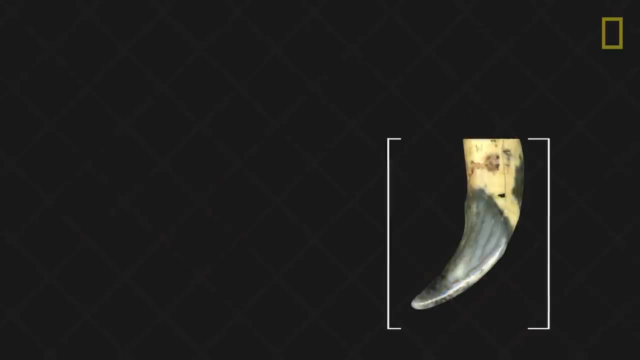 and archaeological evidence suggests that Neanderthals had a relatively sophisticated culture. They built shelters, made and wore clothing and created advanced tools. In fact, they were the first human species to make tools out of bone, not just stone. They also created objects that served ornamental purposes. 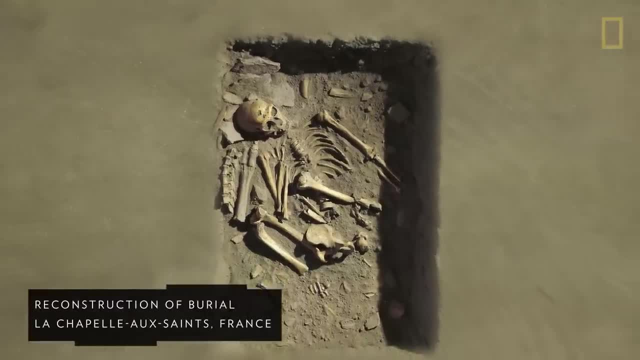 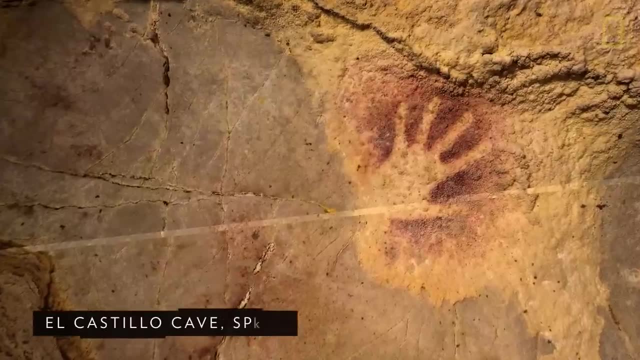 Neanderthals are suspected to be the first humans to carry out the symbolic gesture of burying their dead and adorning gravesites with flowers. Neanderthals may have also created what may be the world's oldest cave art, which was found in Spain. 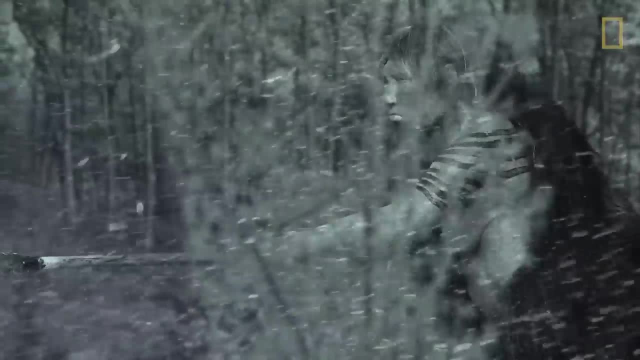 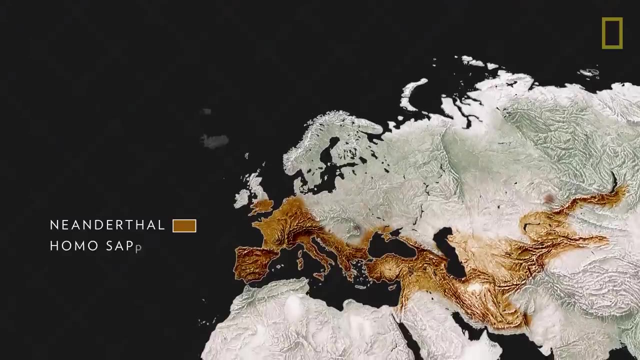 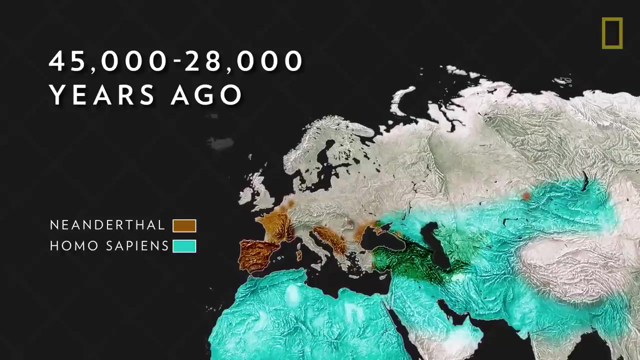 Despite advances in their culture. sometime after 40,000 years ago, Neanderthals mysteriously disappeared. Some scientists believe the Neanderthals were killed or out-competed by modern humans or Homo sapiens who arrived in Europe at around the same time.